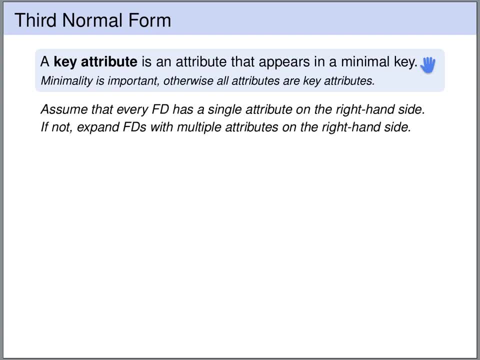 some minimal key For the definition of the third normal form. we assume that we have made all of the right-hand sides of functional dependencies singular. So if a function of dependencies has more than one key, then the third normal form is more than one key, then one functional dependency. then we split this into multiple functional 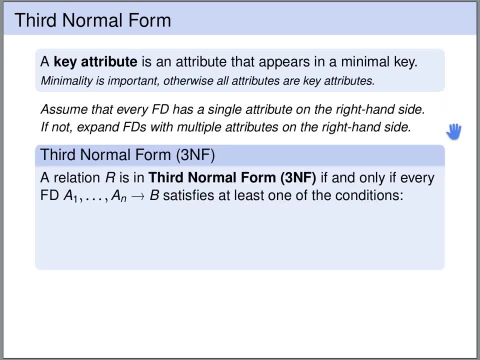 dependencies. A relation r is said to be in third normal form. if for every functional dependency, now with a single attribute on the right, one of the following conditions is satisfied, The first two conditions are just the same as for the Boyce-Codd normal form, Either. 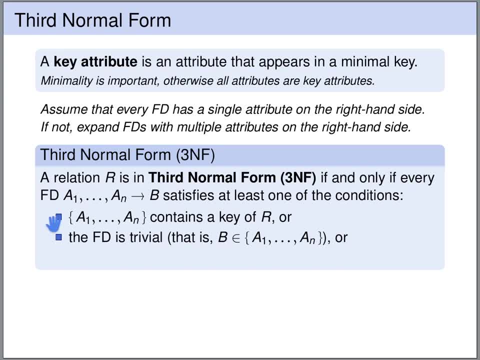 the left-hand side contains a key of the relation, or the third normal form contains only one, Or the function dependency is trivial, meaning that the right-hand side is a subset of the left-hand side. There is one more condition, and this condition distinguishes the third normal form from the Boyce-Codd normal form. 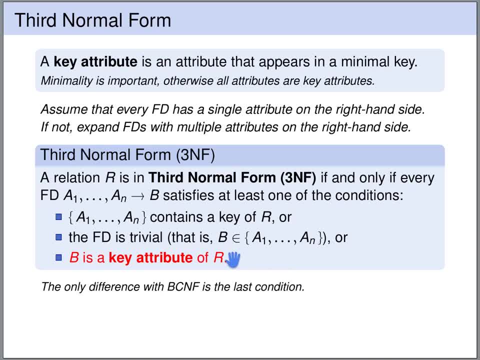 Namely, it is also allowed that the right-hand side is a key attribute of the relation R, And this condition, displayed in red, is the only difference with the Boyce-Codd normal form. So since these conditions are in a disjunction, the third normal form is slightly weaker than the Boyce-Codd normal form. 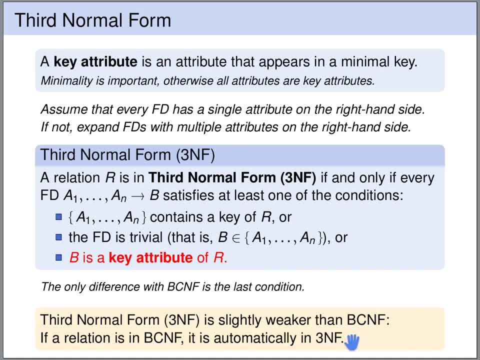 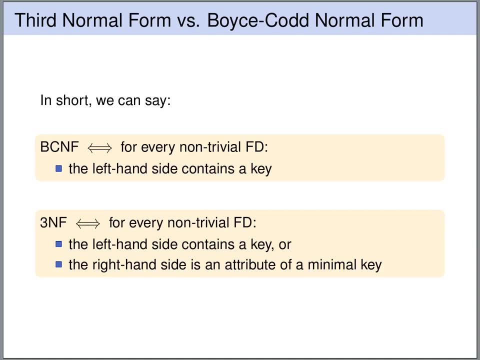 So every relation that is in Boyce-Codd normal form is automatically also in third normal form, But not the other way around due to this additional condition. So, in short, we can summarize Boyce-Codd normal form and third normal form as follows: 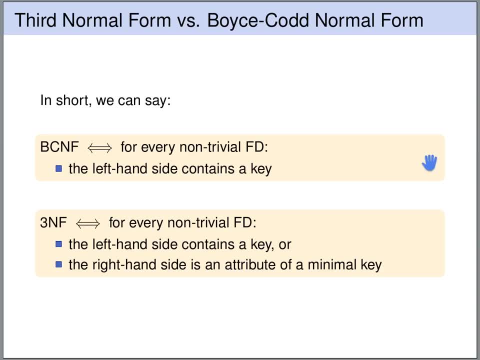 A relation is in Boyce-Codd normal form if, and only if, for every non-trivial function dependency, the left-hand side contains a key. And the relation is in third normal form if, and only if, for every non-trivial function dependency, the left-hand side contains a key or the right-hand side is an attribute of a minimal key. 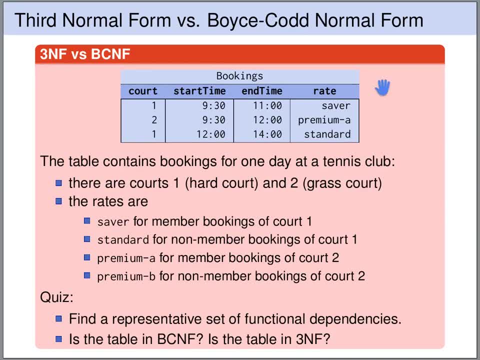 Let's have a look at one more example. Here we have the bookings for a small tennis club. We have only two courts. Court 1 is a hard court. Court 2 is a grass court. In this bookings table we only have the bookings for a single day. 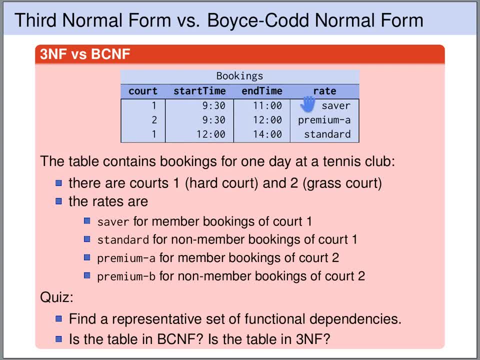 So we have the court number, the start time, the end time and the rate at which the booking has been made. We have different rates. We have the saver rate for member bookings of court 1.. We have the saver rate for member bookings of court 1.. 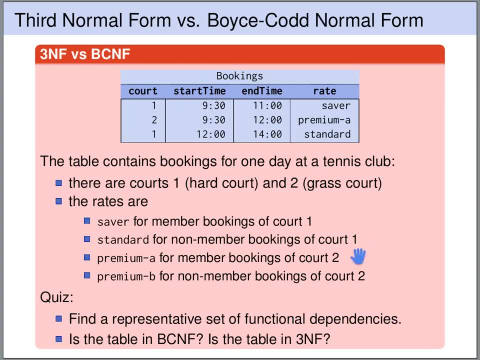 The standard rate for non-member bookings of court: 1.. Premium A for member bookings of court: 2. And Premium B for non-member bookings of court: 2.. Our task is to find a representative set of function dependencies and to decide whether this table is in Boyce-Codd normal form or in third normal form. 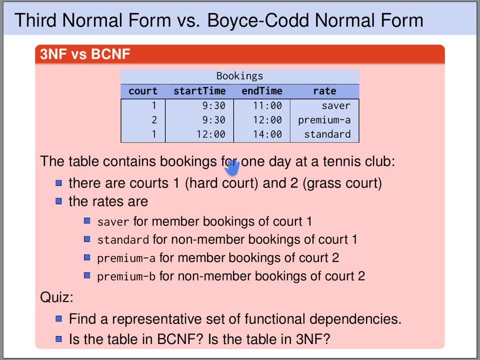 So let's first discuss the representative set of function dependencies. No attribute on itself is a key for this relation. However, the court and the start time together form a key. If I tell you what court and when the booking starts, then you know when the booking will end and you also know the rate. 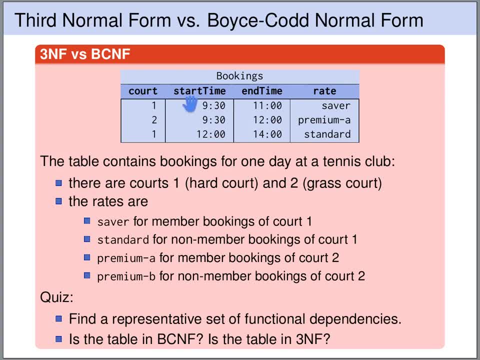 So the combination of court and start time forms a key. They uniquely determine all other attributes. Likewise, the combination of court and end time forms a key of this relation. The combination of court and end time uniquely determines the start time and the rate. 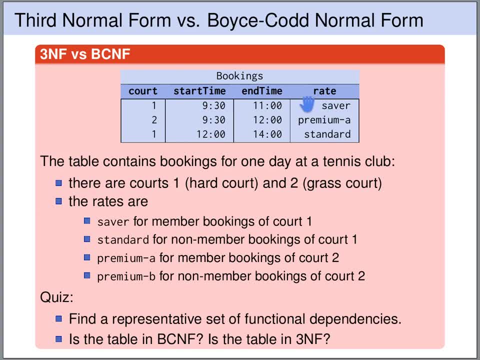 Moreover, the rate uniquely determines the court because we have saver and standard for court 1 bookings and Premium A and Premium B for court 2 bookings. So we have three functional dependencies that imply all other functional dependencies. The first we have court start time uniquely determines end time and rate. 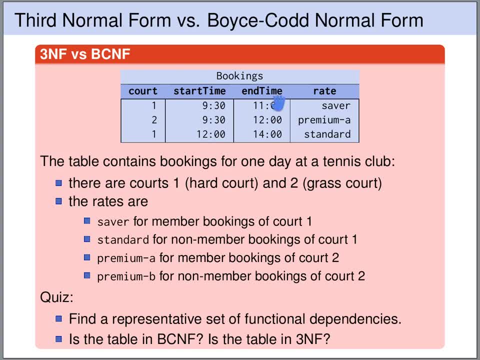 We have court- end time uniquely determines start time and rate. And we have a functional dependency- the rate uniquely determines the court. And these three functional dependencies imply all other functional dependencies. For instance, they also imply that the rate and the start time together form a key. 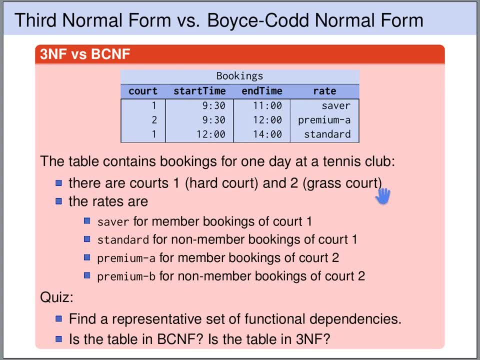 Uniquely determining the court and the end time. So is this table invoice code normal form? No, it is not. If you are looking at the functional dependency, the rate uniquely determines the court. Then the left hand side, the rate, is not a key of this relation.